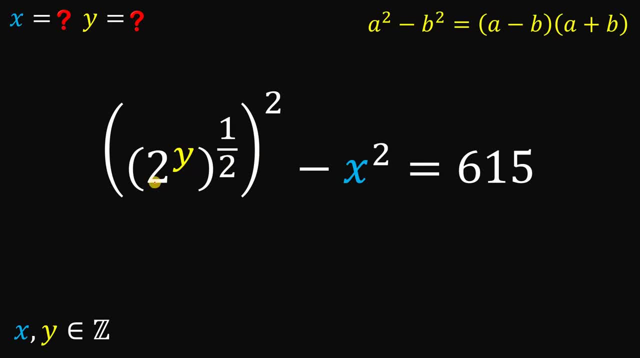 Now 2 times 1 over 2, this is just 1.. So this is simply 2.. Equivalent to 2 raised to y. And now y times 1 over 2, this can be written as y over 2.. 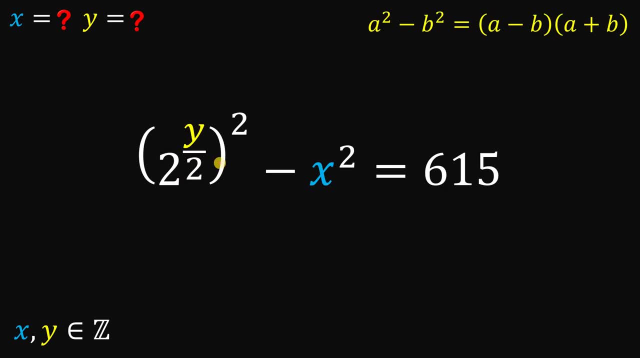 So now 2 raised to y can be written as 2 raised to y over 2 raised to the power of 2.. Now, this is now a perfect square. Therefore, we can now factor the left-hand side as follows: 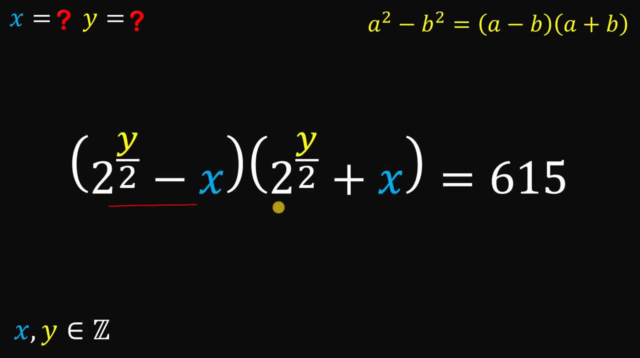 We have 2 raised to y over 2 minus x, Multiply, Multiply by 2 raised to y over 2 plus x, And now let's focus on this number, the constant 615.. Now what we're going to do here is to get its factors. 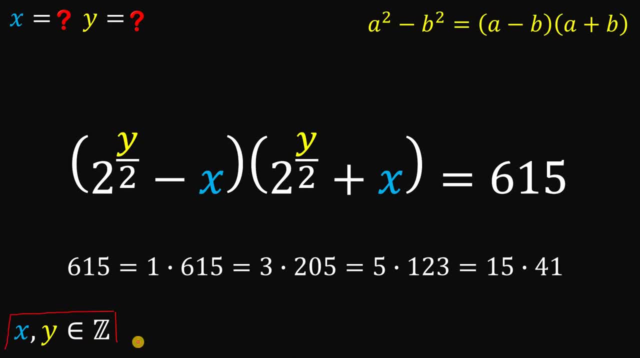 The reason is we are dealing with integer values of x and y. Now, 615 can be factored as 1 times 615, can be factored as 3 times 205.. Right Can be factored as 5 times 123, and can be factored as 15 times 41. 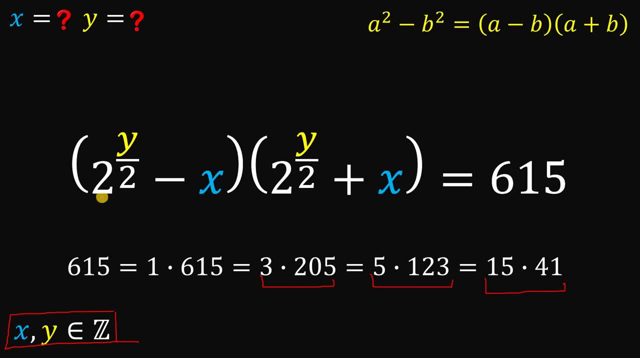 So we can say that 2 raised to y over 2 minus x can be equal to 1. And 2 raised to y over 2 plus x can be equal to 615, and so on and so forth. So to make this calculation more simple, let's make a table of sum. 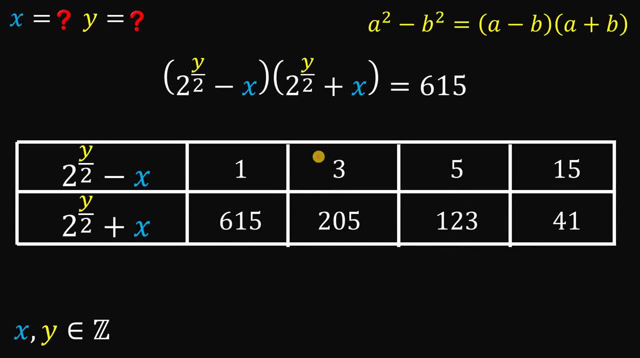 So 2 raised to y over 2 minus x can be 1,, 3,, 5, or 13.. Also, 2 raised to y over 2 plus x can be 615,, 205,, 123, and 41.. 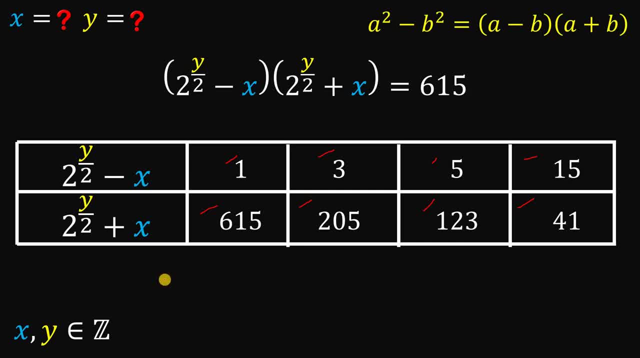 Or vice versa. And now what we're going to do is to add these two equations. And why we do that? Because, take note, when we add these two equations- negative x and positive x- negative x can't sign out. 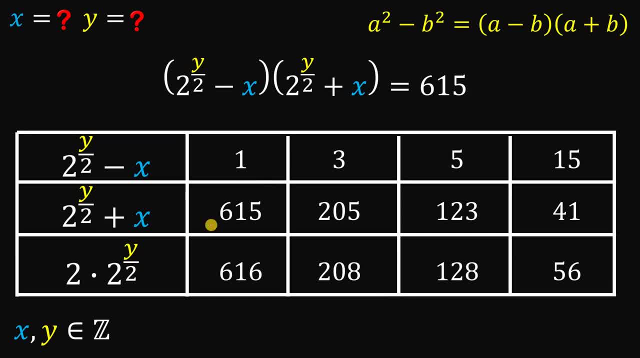 So this will give us 2 times 2. raised to y over 2 must be equal to 1, plus 615 will give us 616.. 3 plus 205 is 208.. 5 times 123 is 128.. 15 plus 41 will give us 56.. 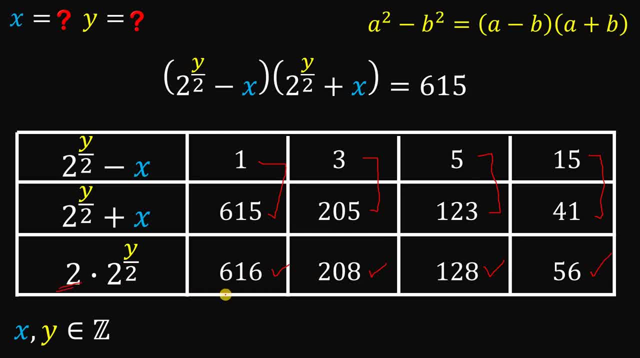 And now we have a lot of factors of 2.. So this is a multiple of 2.. Multiple of 2,, multiple of 2, and a multiple of 2.. So we can divide all of this number by 2.. 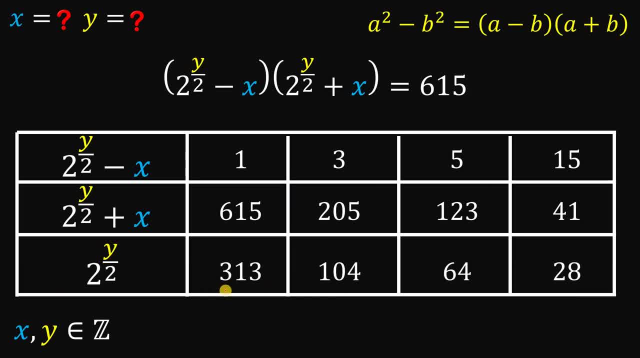 So this will give us 2 raised to the power of y over. 2 must be equal to 313,, 104,, 64, and 28.. Now, 313 cannot be written in 2 raised to some power. So this is not possible. 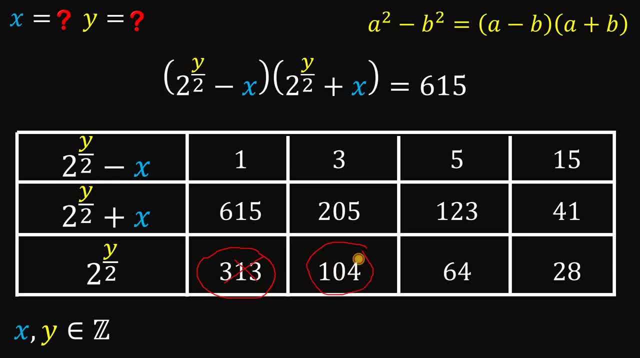 104 cannot be written in 2 raised to some power. This is not possible also. And this 28 cannot be written also as 2 raised to some integer power. But 64 can be written as 2 raised to the power of 6.. 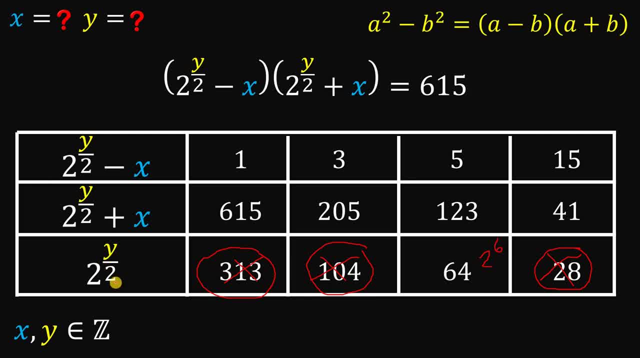 So we have only one possible case here. So 2 raised to y over 2 must be equal to 64. Again, 64 can be written as 2 raised to the power of 6.. Now, since 2 raised to the power of 6 must be equal to 64,, 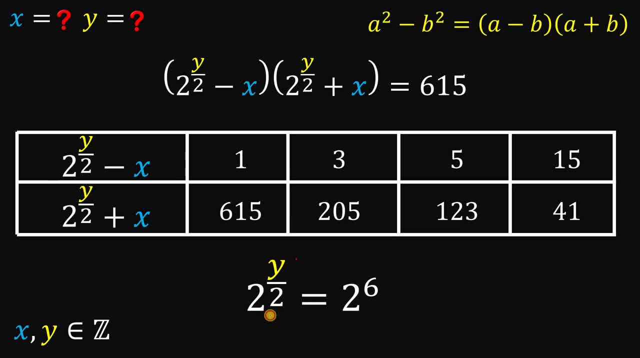 they are equal and the base are equal. So we can say that their exponent must be equal. So we can say that y over 2 must be equal to 6.. Now let's solve for the value of y. Let's multiply both sides by 2.. So we have 6 times 2 will give us 12.. So the value of y must be equal to 12.. Now how? 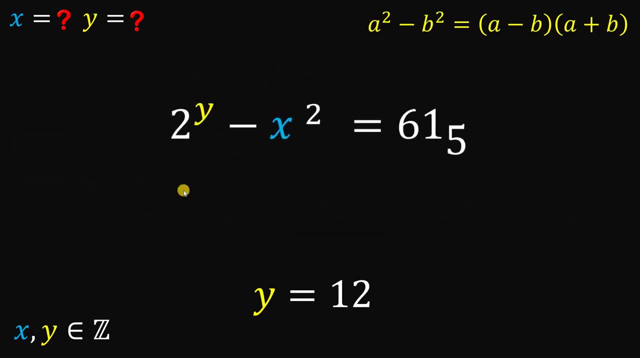 about the value of x. Let's go back to our original equation. So we have 2 raised to y minus x, squared equals to 615.. We now know the value of y. This is equal to 12.. So we can replace this y with 12.. And 2 raised to 12 must be equal to 4096.. Now let's solve for the value of x. 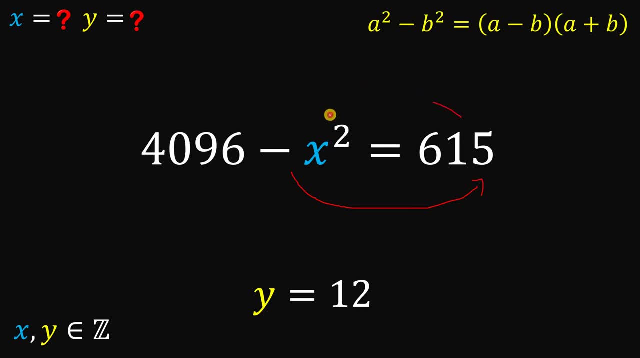 Let's add x, squared on both sides, and let's subtract 600.. Now for 1096 minus 615, this will give us 3481.. Now we want to solve for the value of x. So let's get the square root on both sides. Now we have two possible values here. We have positive or